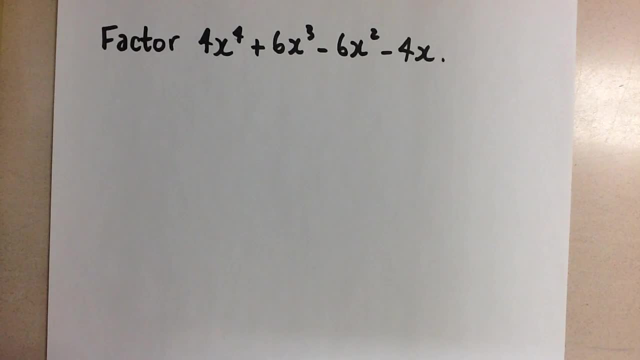 Hi guys. Mrs A, here We are looking at factoring polynomial functions of a degree higher than 2.. We know how to factor quadratics. You can look back at my other videos if you need a refresher on that. But now we're going to look at factoring this polynomial and the degree of this polynomial. 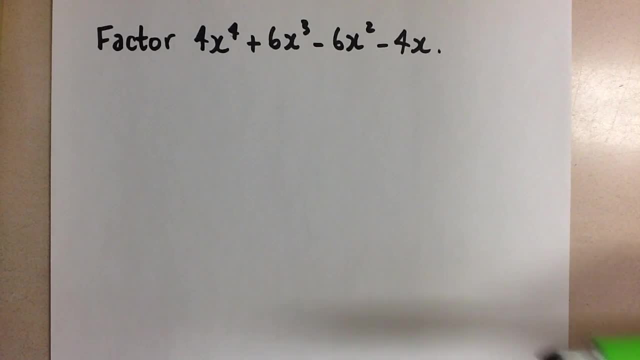 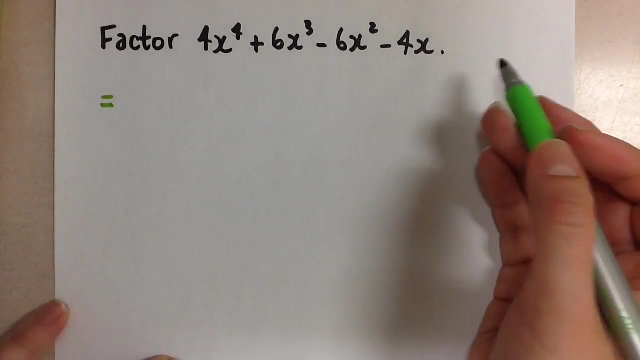 is 4.. So the steps for factoring this are a little different than just a quadratic or a polynomial of degree 2. The first thing we always, always look at is if we can take out a common factor. So in this case, when I look at all of my terms, I see that I have a common factor. 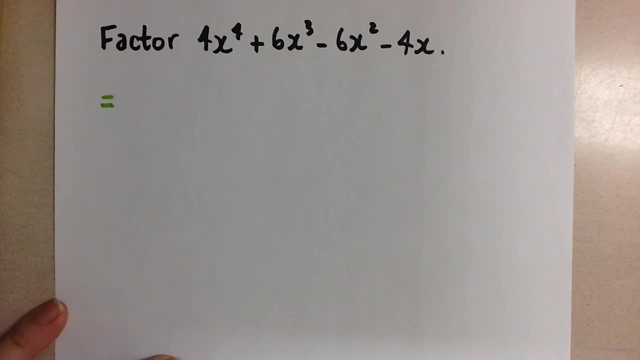 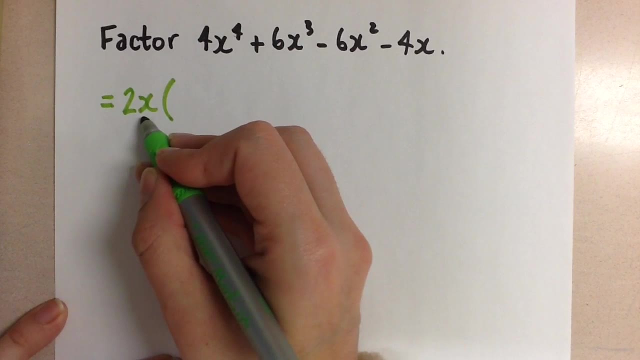 here of 2x. So that's the first thing I'm going to do. It simplifies the expression and makes everything a little bit easier. So if I pull out a 2x from every term, I'll have a 2x cubed. 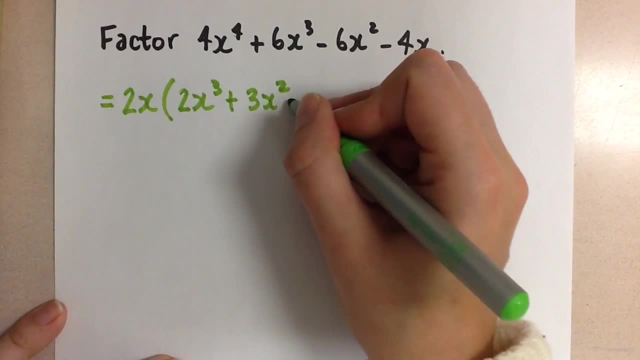 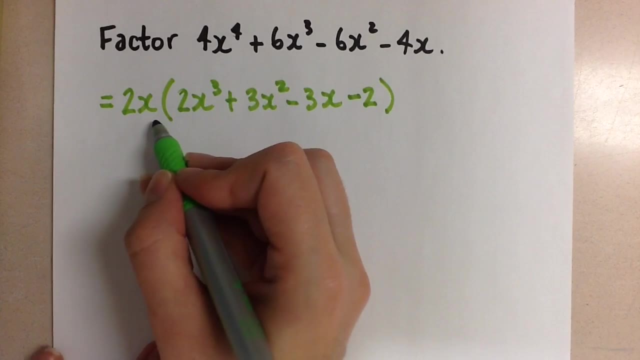 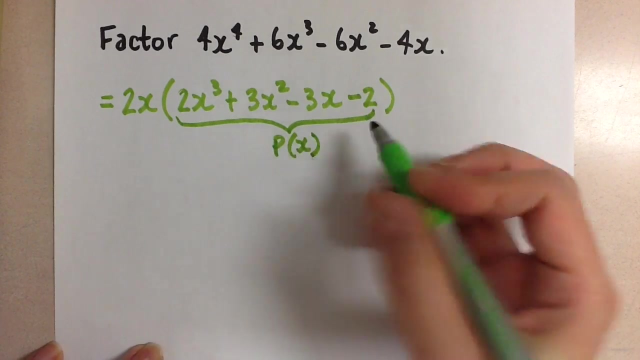 plus 3x, squared minus 3x minus 2.. This 2x we're going to leave as one of the factors for our final factored expression, And now we're going to concentrate on just this portion in the brackets. We'll call this the new polynomial that we want to factor. So we've reduced it now to a 3 degree. 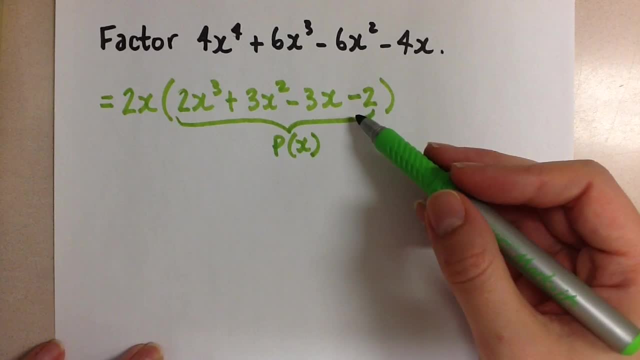 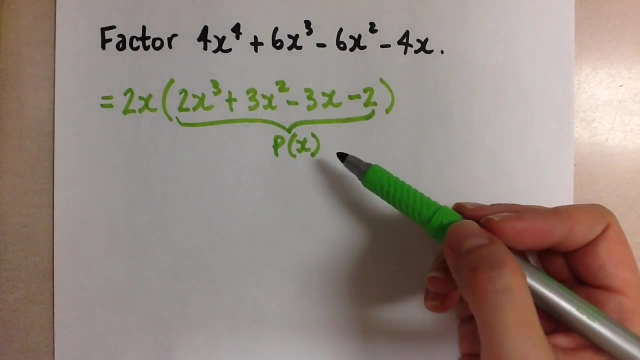 polynomial that needs to be factored. So let's call this the new polynomial that we want to factor. We'll call this: p at x. In order to factor this, we have to make use of the factor theorem. The factor theorem says that if x minus a is a factor of the polynomial, then the remainder 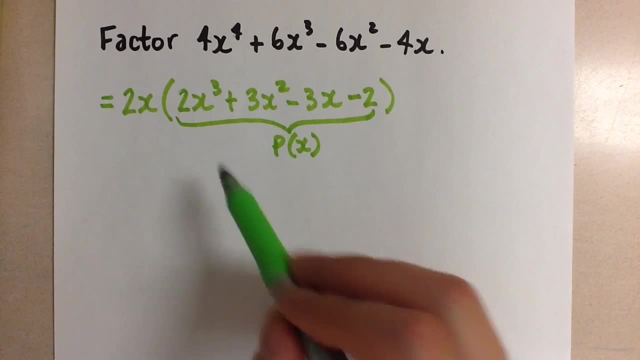 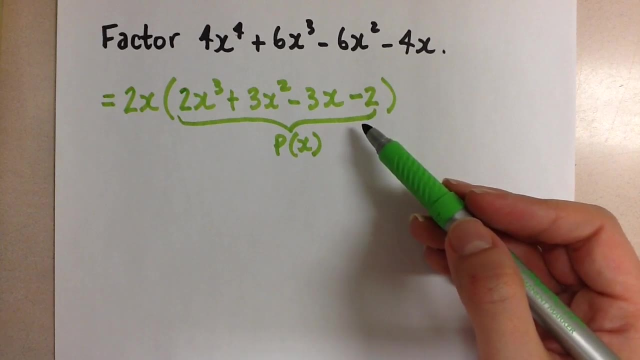 is going to be equal to 0. We know that we can find the remainder of any polynomial using the remainder theorem. So if a factor is 0,, we can find the remainder of any polynomial. So if a factor is 0,, we can find the remainder of. 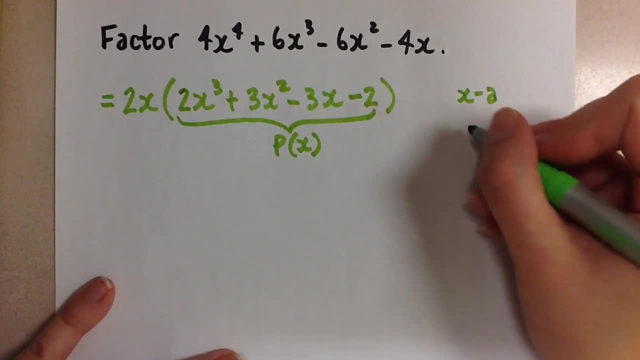 any polynomial. So if a factor is 0, we can find the remainder of any polynomial. So if the divisor is x minus a, then p at a is going to be equal to the remainder. So if x minus a is a factor, then our remainder is going to be 0. 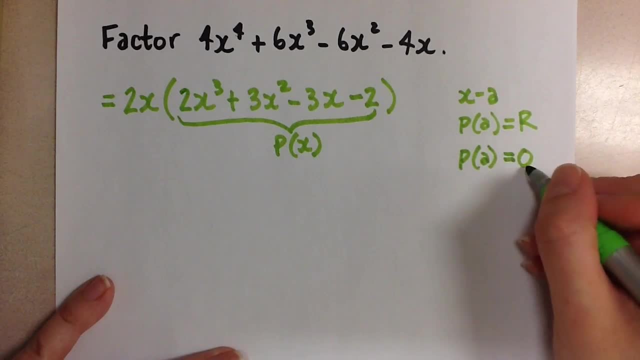 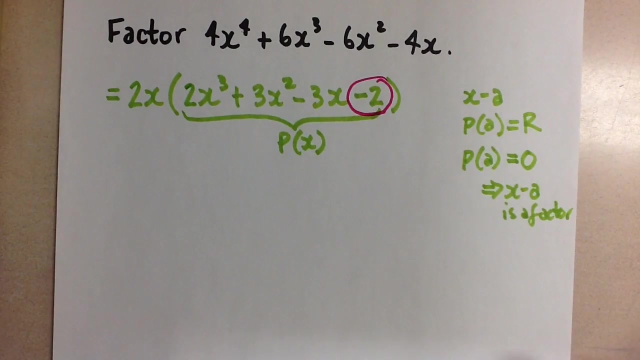 So we're looking for the, a value that makes the remainder 0, and that will tell us that x minus a is a factor. To do that, we're going to look at the last constant constant term of the polynomial, and the factors of that number are what's going to lead to. 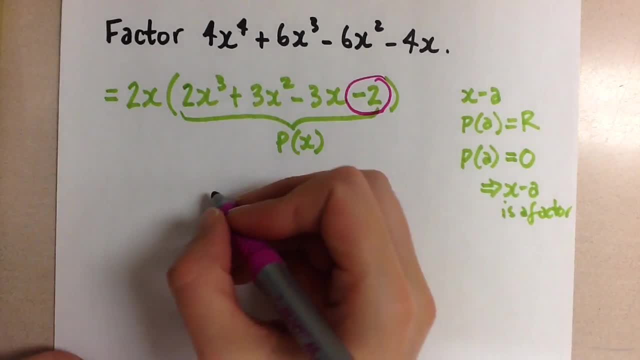 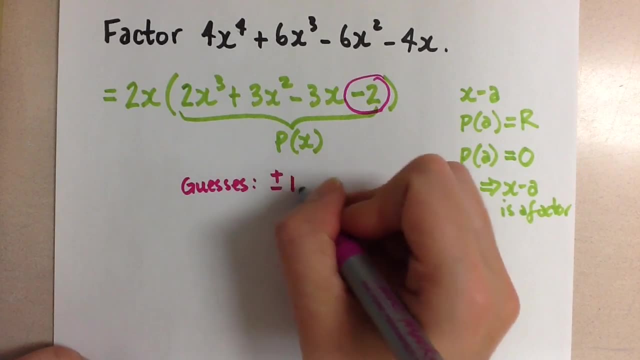 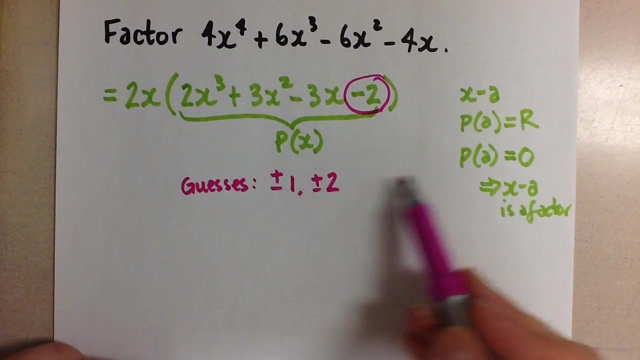 the guesses for this divisor that we're looking for. So the factors will be our guesses, and they are positive and negative 1, and positive and negative 2.. So we start subbing in these values until we get a remainder of 0.. 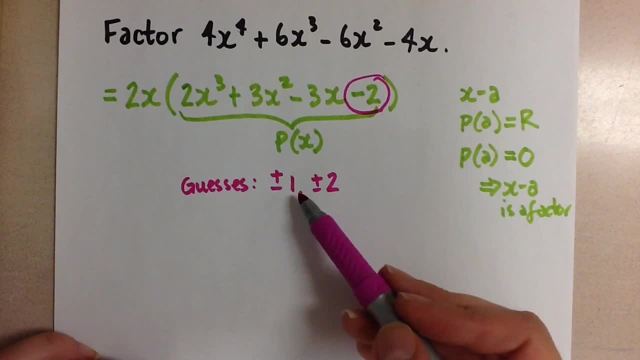 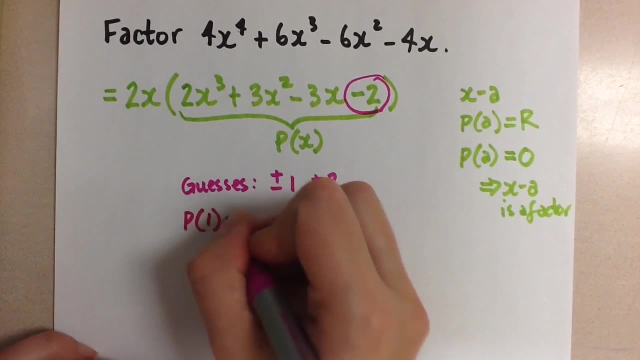 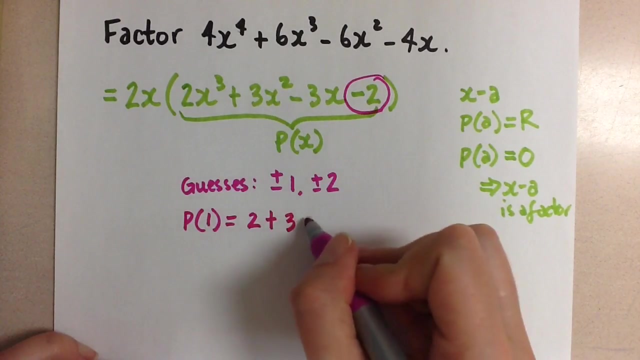 I always recommend that we start with the simplest number, and that is always positive 1.. If I sub in positive 1 here, we'll get 2 times 1, plus 3 times 1, minus 3 times 1, and then 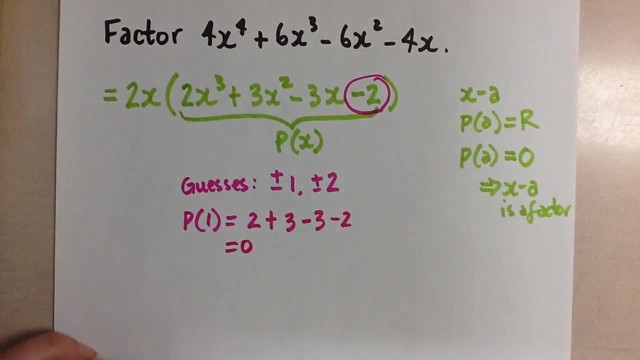 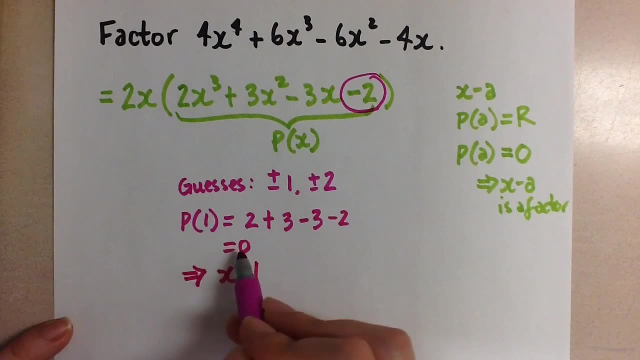 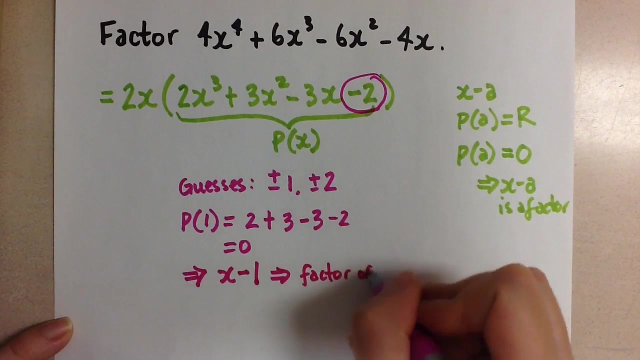 minus 2. And that is equal to 0. So this means we found it on our first try, x minus 1, because p at 1 is equal to 0. This is a factor of the original polynomial we were dealing with. 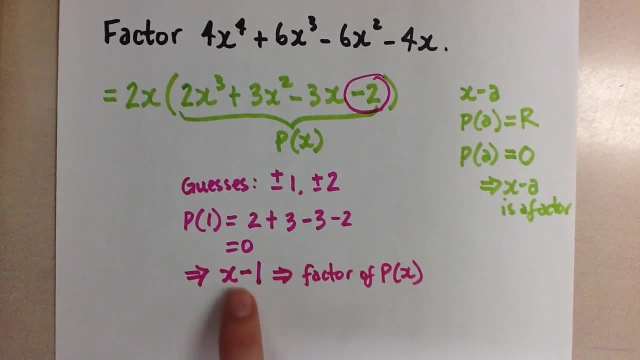 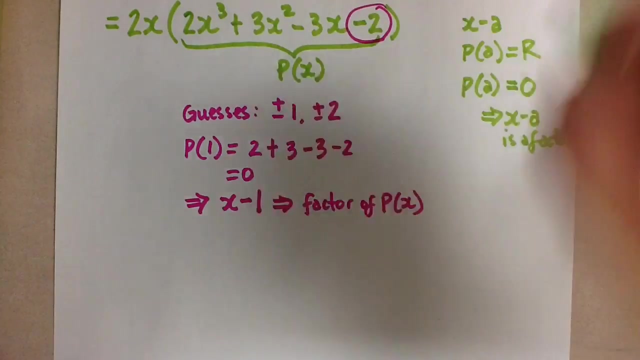 There. So if we know it's a factor, we know that we can divide x minus 1 into that polynomial and we should get a remainder of 0.. And then the quotient… The quotient will be the other factor. So let's go ahead and do that long division. 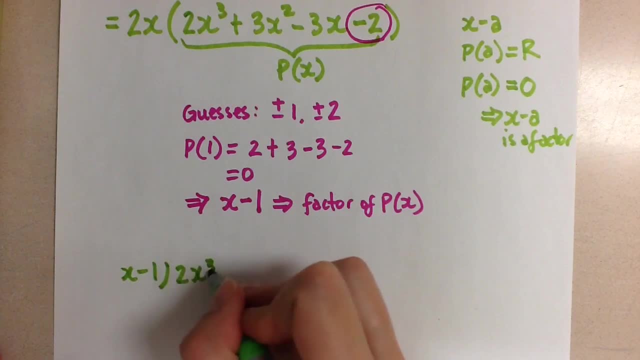 x minus 1 into 2x cubed plus 3x, squared minus 3x minus 2.. And we'll do the long division here quickly. If you need to remind yourself of the long division of polynomials, then go to my previous. 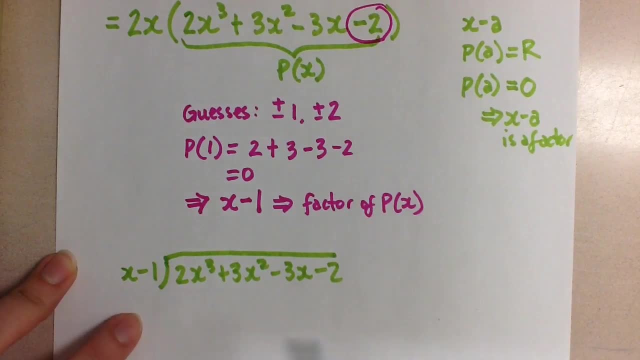 video. I'll link to it here And you'll see this process in more detail. So x goes into 2x cubed, 2x squared times, and we get 2x cubed here. When we multiply, we get minus 2x squared. Subtract The first two cancel And here we have 5x squared minus 3x And we get 2x Subtract 3x. x goes into 5x squared 5x times. We multiply and get 5x squared minus 5x.